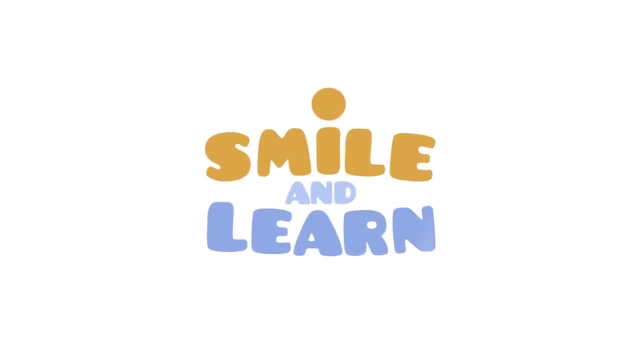 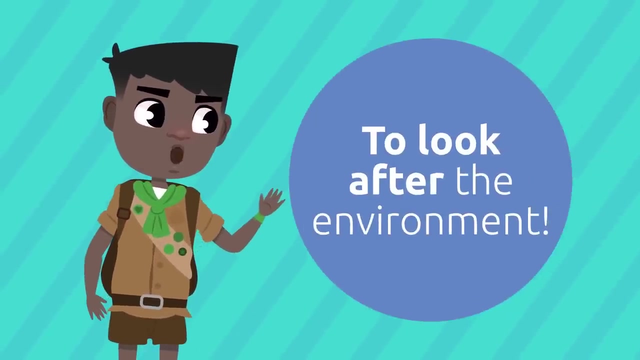 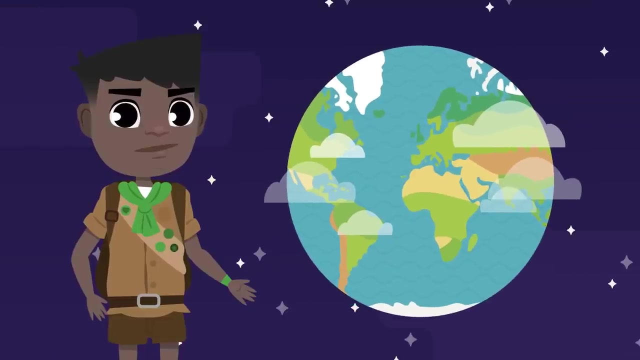 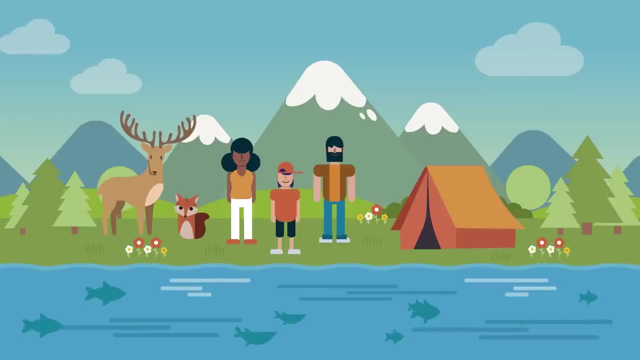 Hey there, friends, I have a very important mission: To look after the environment and help so that kids like you join us in this task, which is vital for our planet. As you may already know, human beings and the environment are closely linked together. Every time people 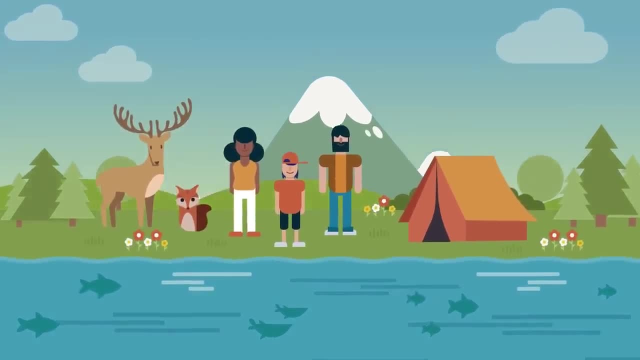 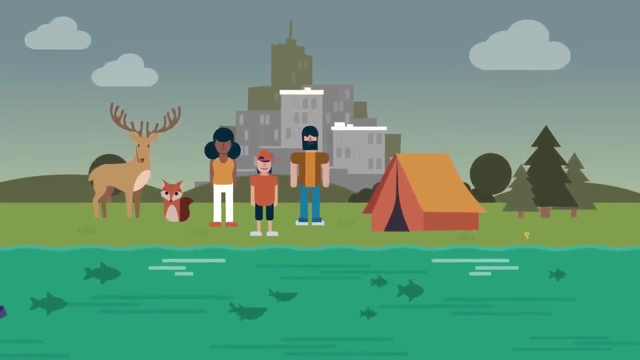 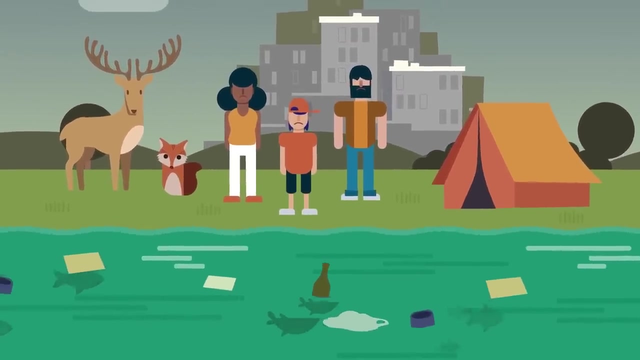 harm nature, they cause environmental problems. These problems involve damaging changes in the environment, many of which will be irreversible and will affect the health of all human beings. Look at this river. People have thrown waste in it, the water has been contaminated and 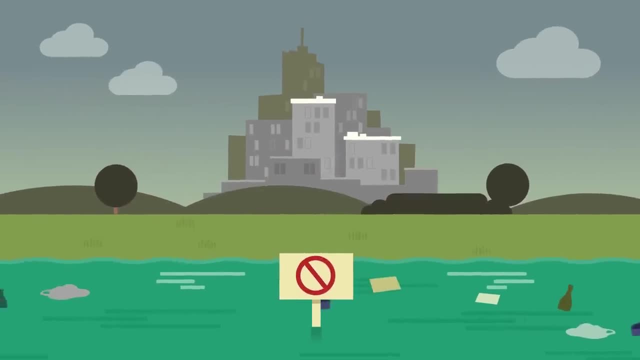 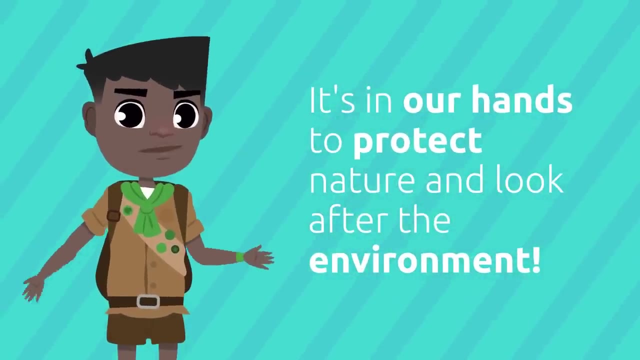 now, nobody can drink it. Oh no, There are also many animals and living beings that will die because of contamination. Luckily, it's in our hands to protect nature And look after the environment. That's why I want to share with you these 10 easy ways. 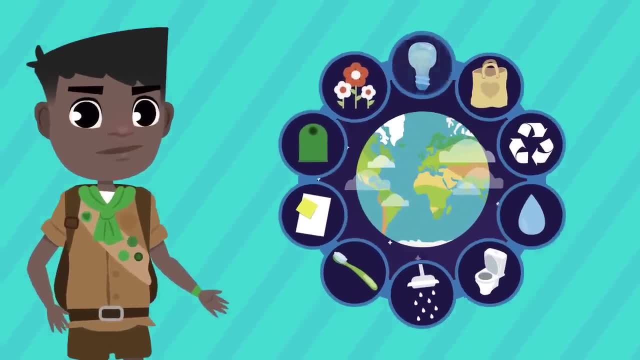 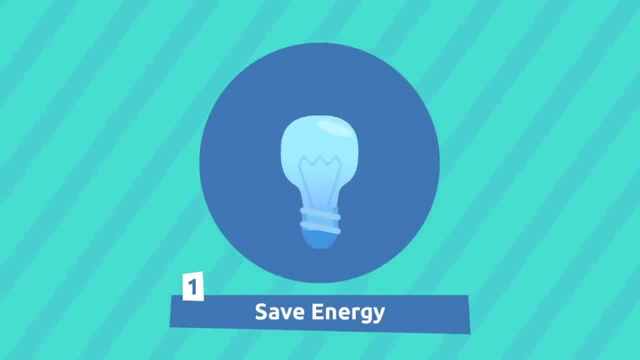 to look after the environment. Let's take a look. Turn off the lights and the electronic devices you're not using to save energy. Replace plastic bags with reusable cloth bags. It takes plastic bags years to decompose and making them is a very contaminating process. 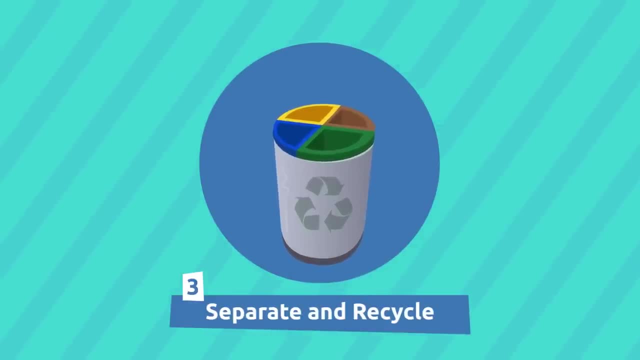 Separate and recycle the different types of waste: Organic, inorganic containers, glass or paper and cardboard. To avoid wasting water, make sure taps are completely turned off. The toilet is not a rubbish bin. Did you know that we waste 10 liters of water every time? 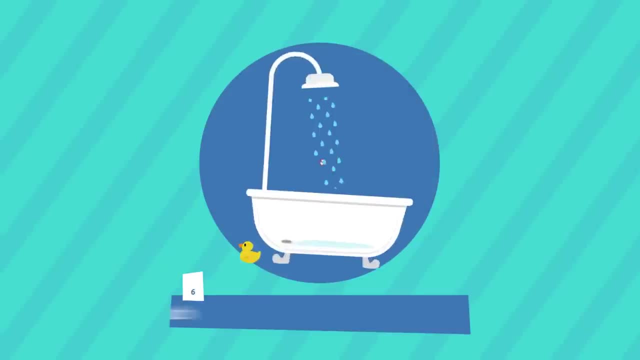 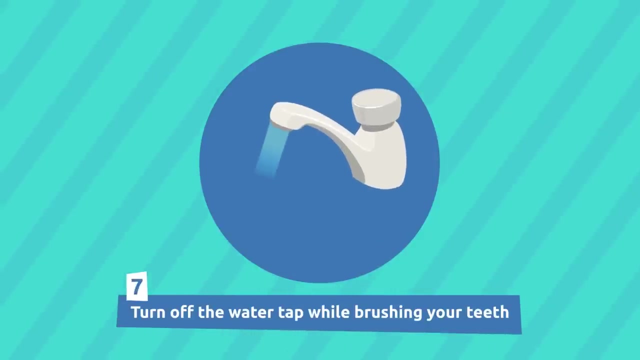 we flush the toilet. Have a shower instead of a bath. A five-minute shower uses about 100 liters of water, while a full bath would use up to 250 liters. Turn off the water tap while brushing your teeth, If you didn't shut off the faucet.